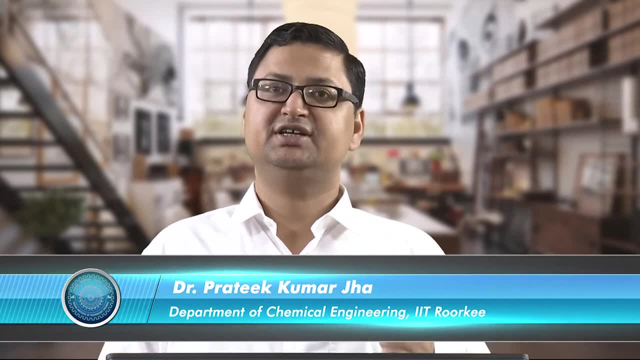 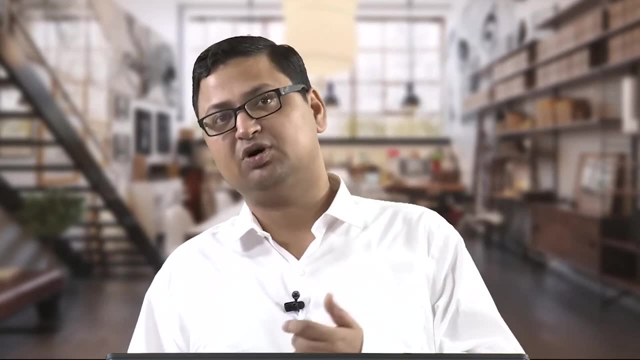 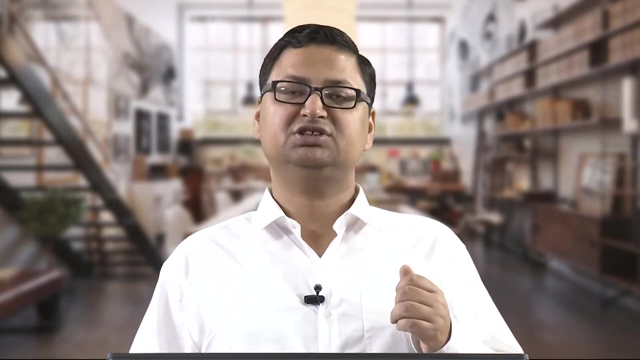 in general. we will then apply to the models of polymer chains that we have discussed, the particularly the bead spring model, and what we will develop is then called the Rouse model. that is used to find the diffusion coefficient of polymer chains, and after we have finished doing the Brownian motions in the next couple of weeks, we can go on and talk about the behaviour. 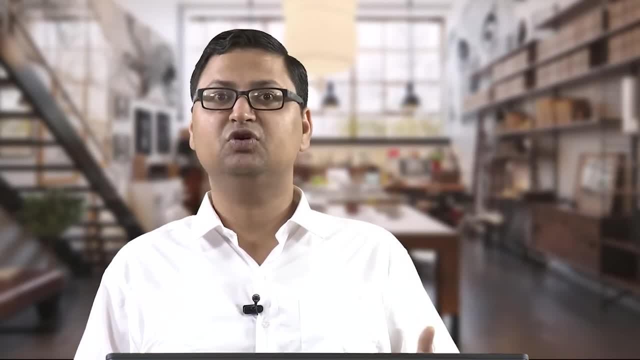 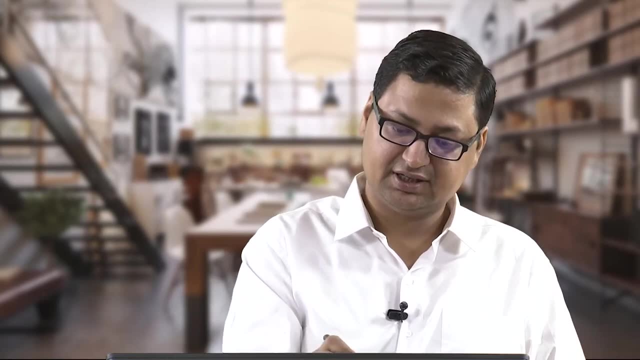 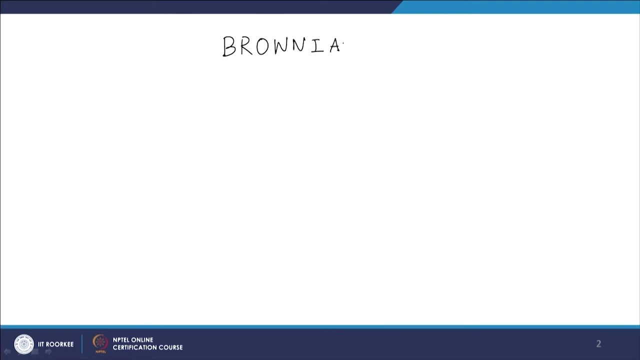 under non-equilibrium cases, the behaviour under flow, and that goes in the subject of rheology. So let us first begin with the concept of Brownian motion and, again, as I have been doing, I will first discuss the concept in general for any system and then we can extend the. 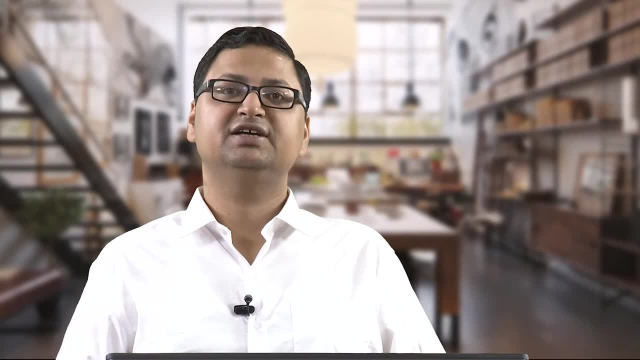 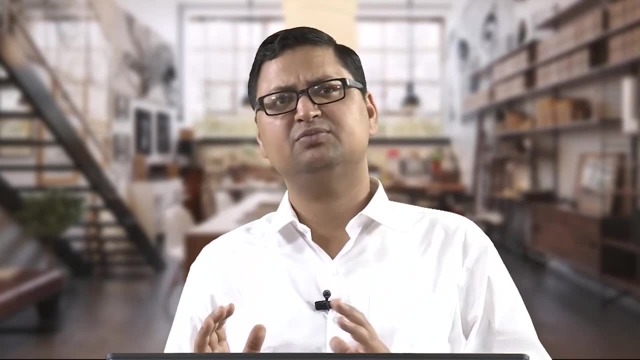 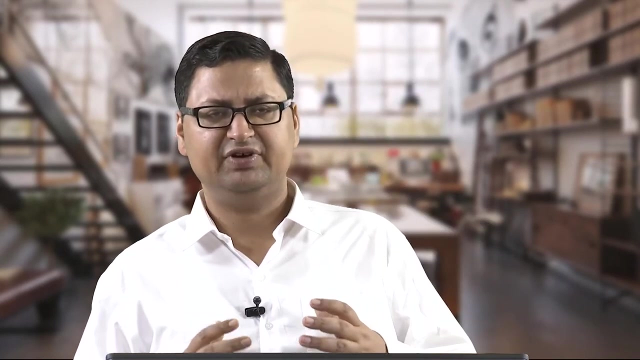 idea to a polymer solution And we will see, like, how the 데ohydrogen origin turns out to be. So if you think of, like what the origin of Brownian motion is, ultimately it is a result of the thermal fluctuations. but even before that, if we start thinking of, like what does the motion of molecule in? 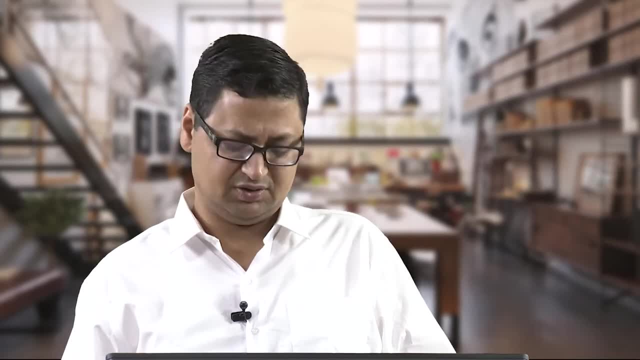 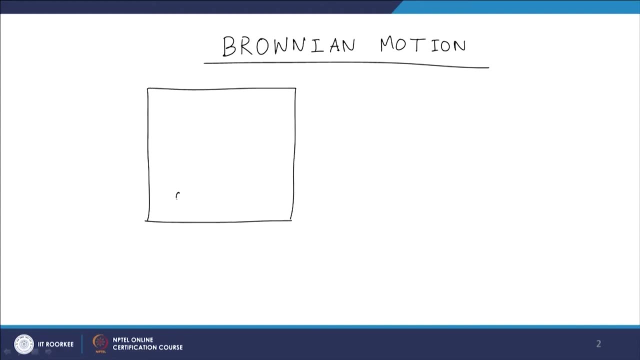 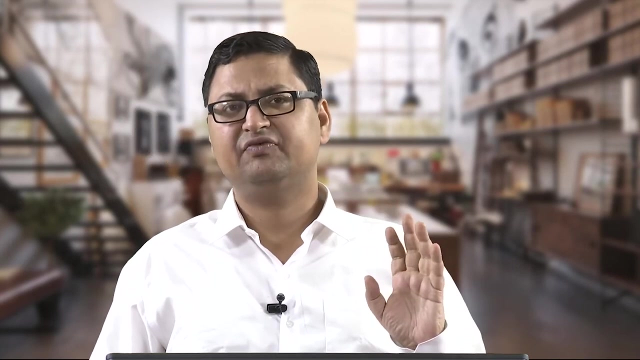 at a molecular level. what do you mean by the motion of molecules? So, for example, if we have some molecules which are present in a beaker or any volume, how will these molecules move? let us say, if I apply a force on the beaker, the force will not result in the collective. 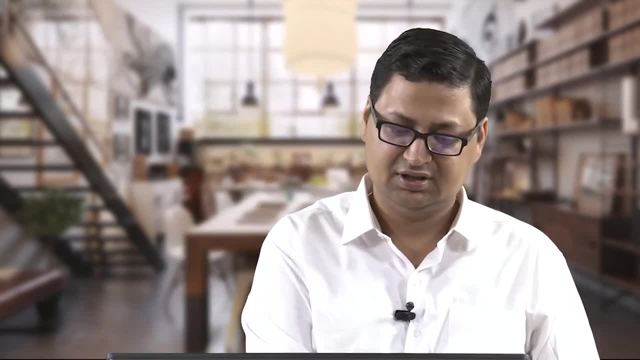 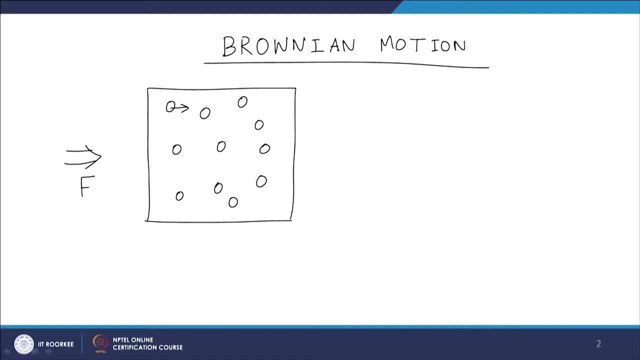 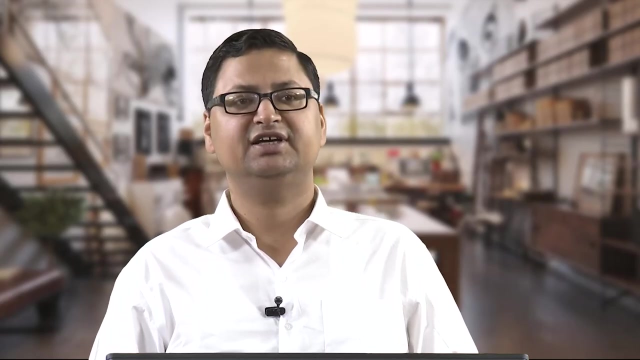 motion of all the molecules in the same direction. that is, if I apply, say, a force in this direction, it would not be that all the molecules would start moving in the direction of the force, as we normally think in the case of a like macroscopic system. let us say, if we have a 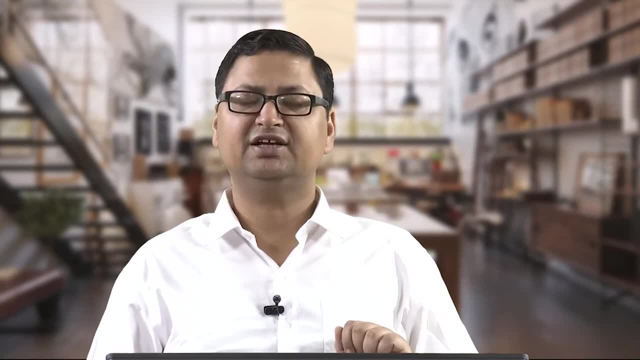 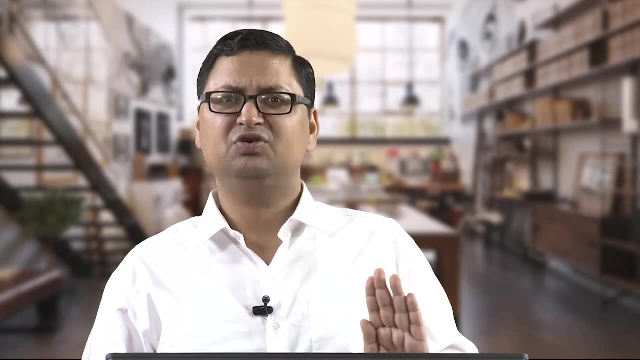 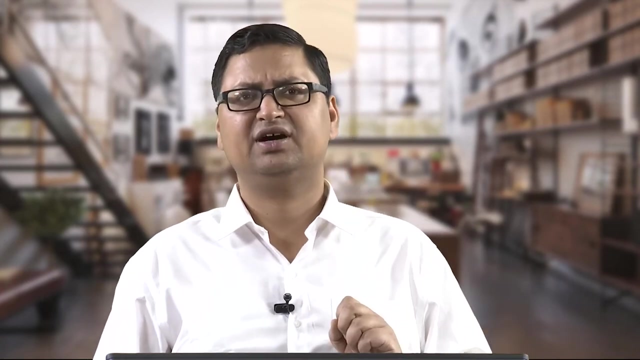 block. I apply a force, the block moves in the direction of a force applied. but if I look at the molecules within the block, they do not quite move in the direction of the force. they actually have what is known, said and some diffusive motion and some convective motion. Of course, if I take an average over many, many of 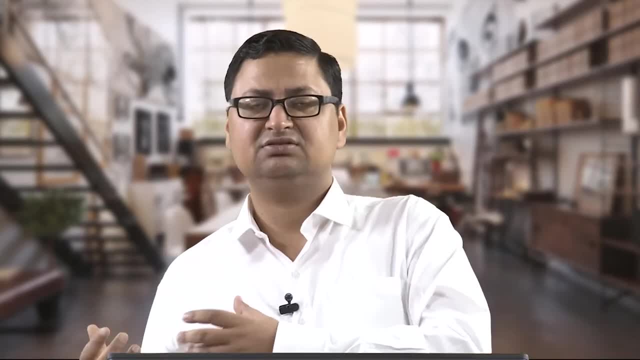 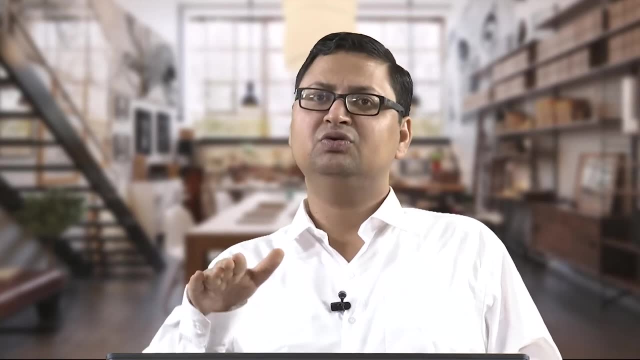 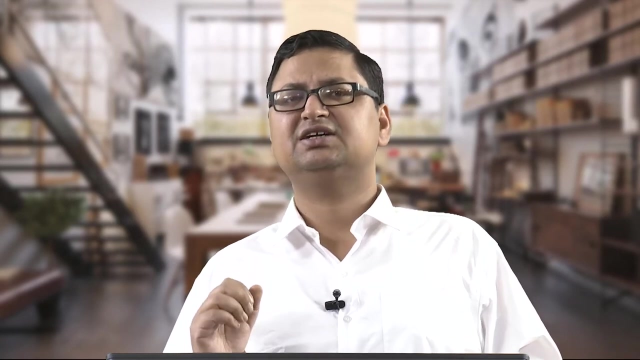 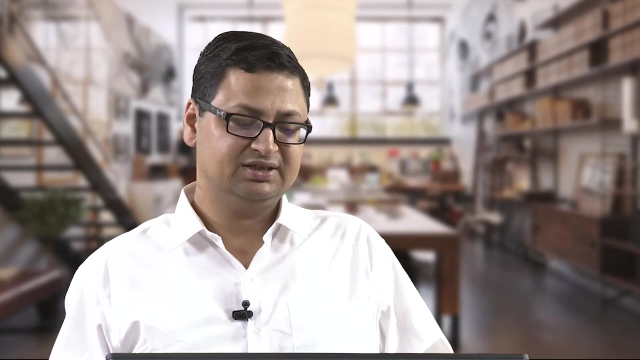 those molecules, what we call a fluid packet in the case of fluid mechanics. then we can assign an average velocity that would be in the direction of flow, direction of the force applied. but individual molecules will actually be having somewhat erratic kind of movement, And such erratic movement are even present when the force is not being applied, even if you have. 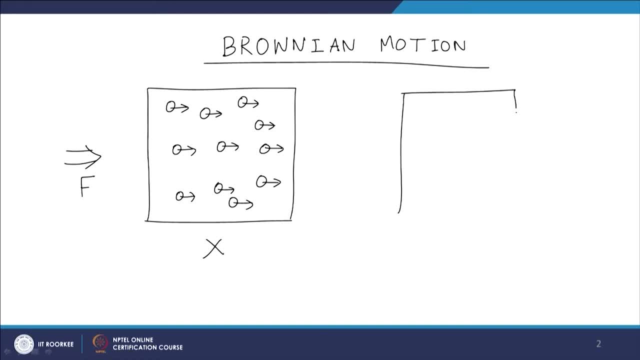 say stationary beaker, particularly liquid, containing different molecules, which I am drawing by circles here. even when the force is equal to 0, even if it is a static or in a state of equilibrium, It is not that the molecules are not moving. Molecules do indeed move, but the motion of molecules are in different directions, which? 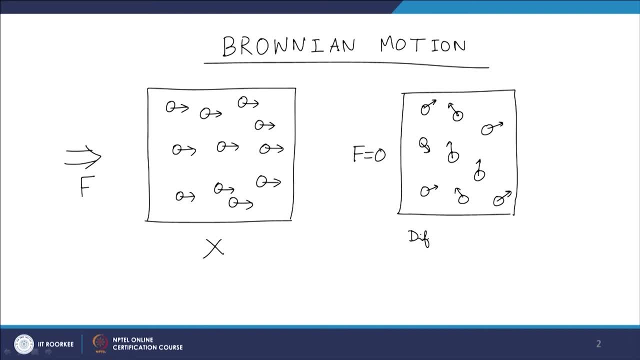 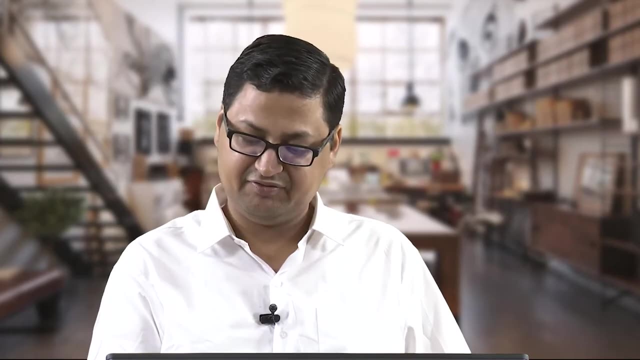 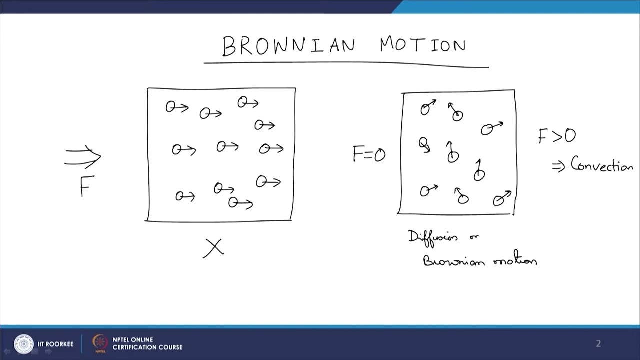 we refer to as diffusion or Brownian motion, and only when an additional force is applied. if the F is higher than g, Then we also have an additional convection. that occur because, on an average, the molecule tend to move in the direction of the force. 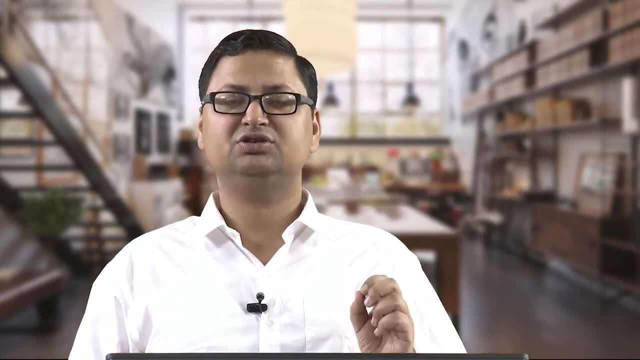 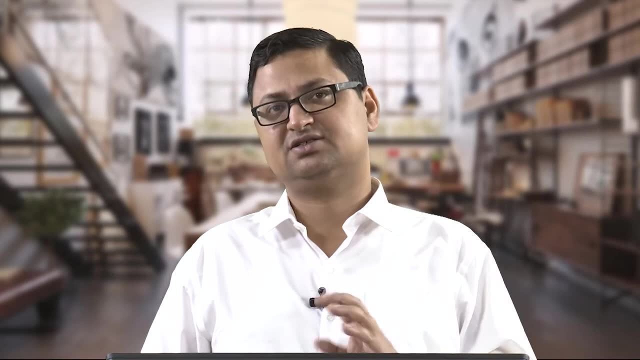 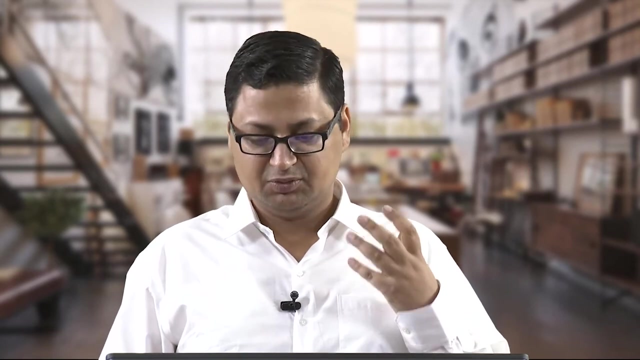 So the first thing to note here is, when we talk about the motion of molecules, it is very different compared to the motion of macroscopic objects that we have been used to seeing. and the reason why it is different? because the motion at the molecular level is dictated. 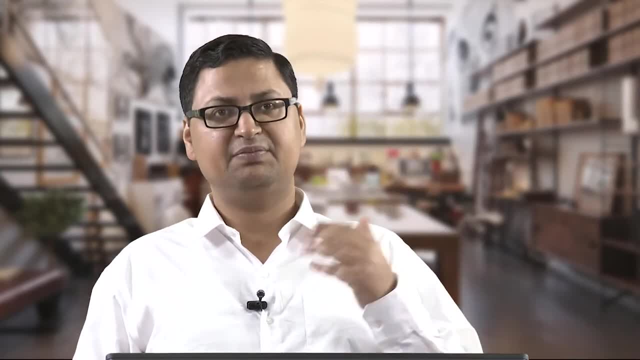 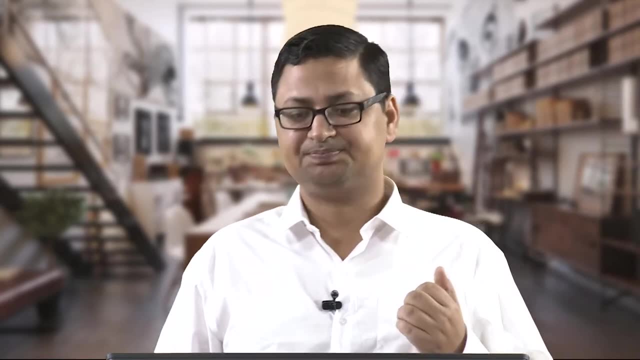 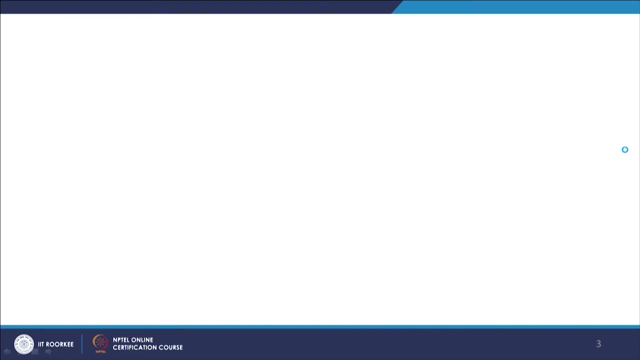 by the kinetic theory or the temperature of the system, And I would show in a moment that why we do not care about that when we go to a macroscopic system. So if you recall from high school the definition of temperature, the temperature of a system, 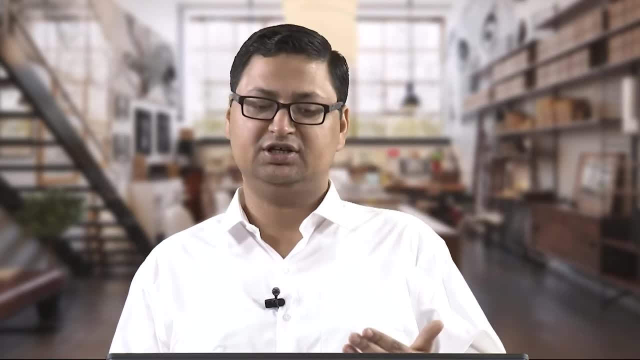 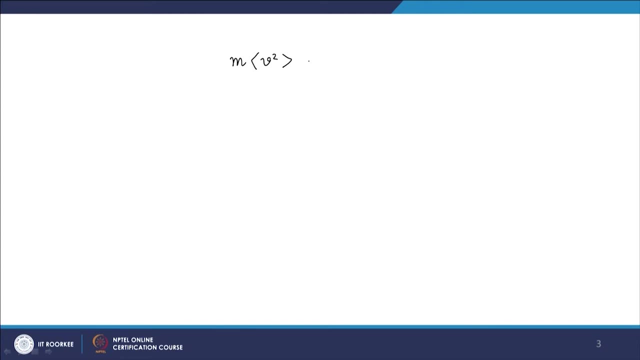 is actually a result of the kinetic energy. So if you recall from high school the definition of temperature, the temperature of a system is actually a result of the kinetic energy And there is an equipartition principle that basically relates the kinetic energy to the 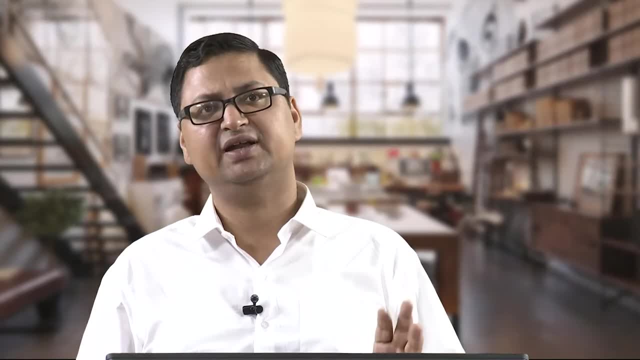 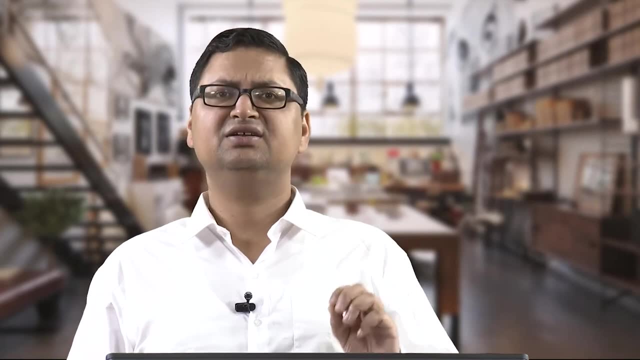 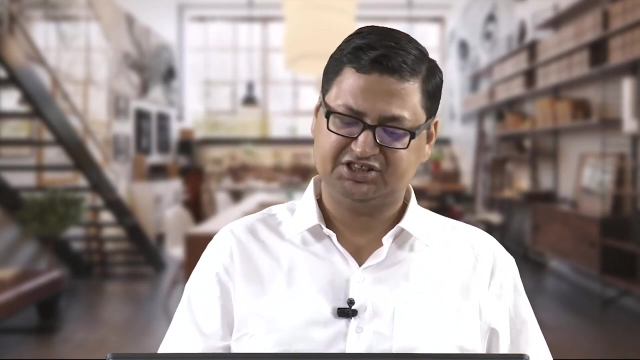 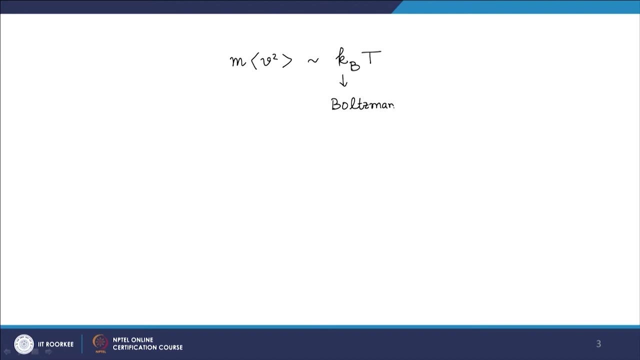 temperature. I am not worrying about the pre factors here. the pre factors vary depending on whether the molecule is monoatomic, diatomic and so on. But in general the kinetic energy is scales like KBT, where KB is the Boltzmann constant and T is a absolute temperature in Kelvin and the Boltzmann constant is of the order. 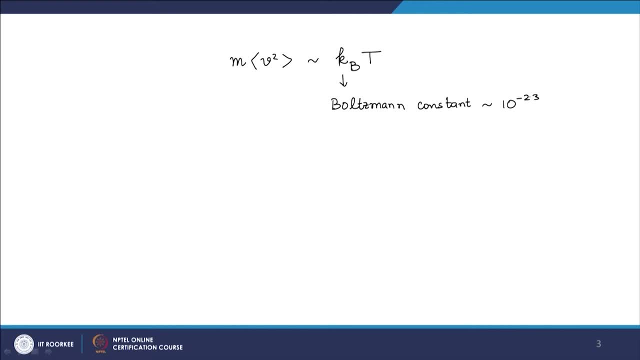 of 10 to the power – 23 in SI units. actually it is joule per Kelvin, because this has a unit of energy and this is in Kelvin, So Kb has to be in joule per Kelvin SI units and temperature typically is of the order of 100. like 300 Kelvin is a room temperature. we typically 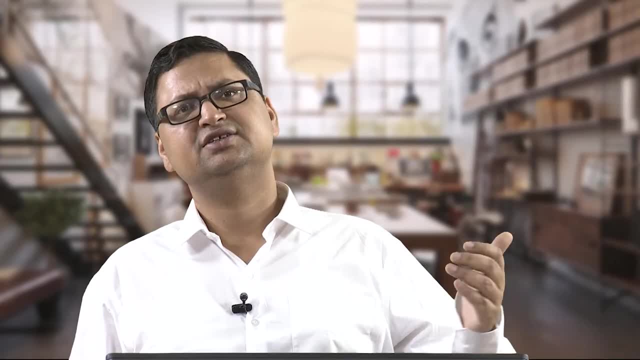 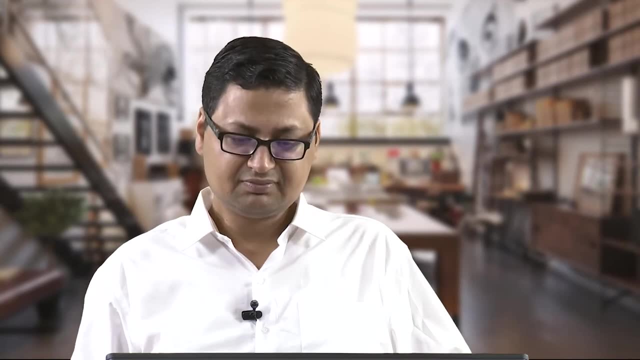 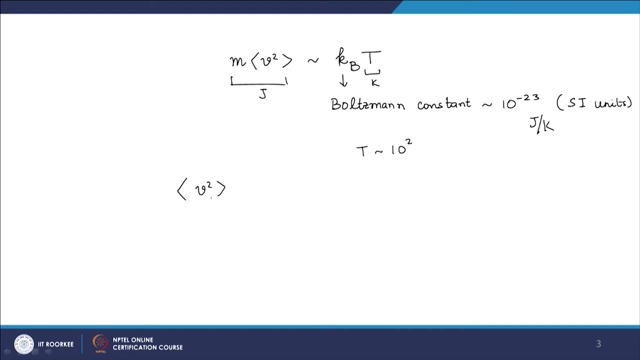 do not go very high in the case of a liquid. but we can go say 500 Kelvin, 16 Kelvin and so on. All of them we can say are of an order of magnitude of 100. So if we then find the mean square velocity of molecules, this goes like kbt by m and so 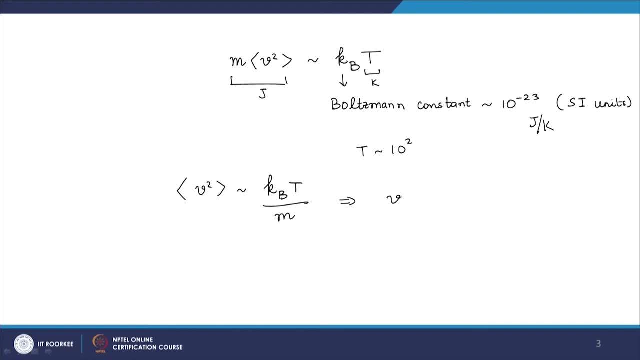 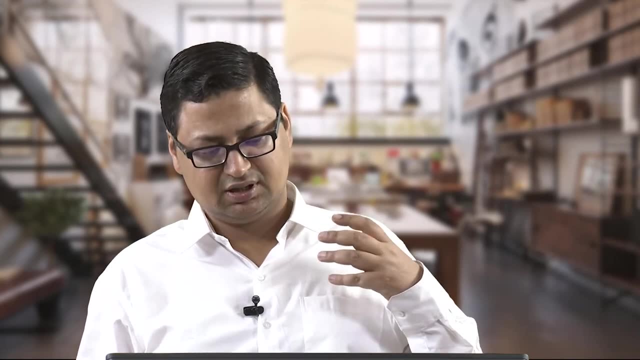 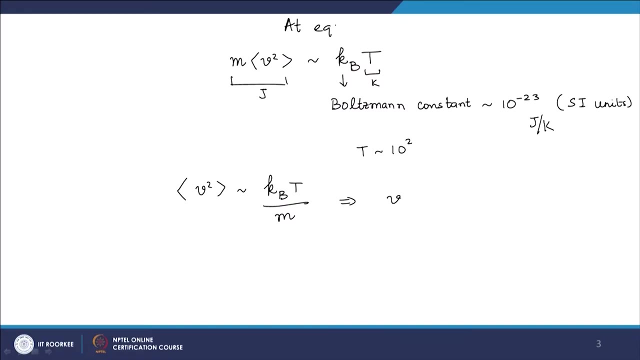 very roughly speaking, the velocity of individual molecules because of the temperature or the molecules velocity that give rise to temperature at equilibrium. So this is without convection. the typically scale like something like kbt by m. okay, And now let us try plugging in numbers here and try to see like how much this velocity. 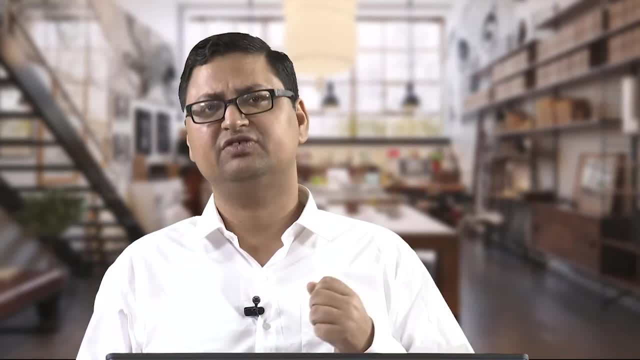 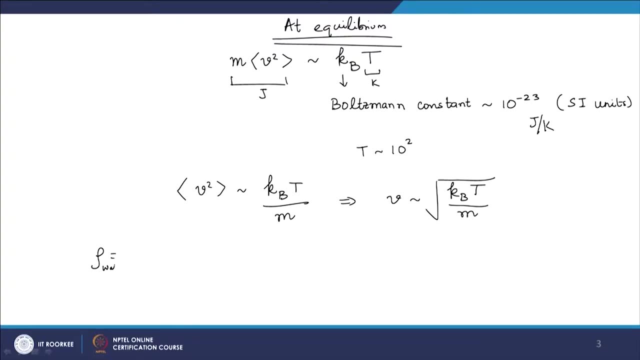 is for particles of different size or molecules of different size. Let us just know that the density of water is 1 gram per centimeter cube and so if I have, say, a block of 1 centimeter in each direction, a cubic block, it will have a volume: 1 centimeter. 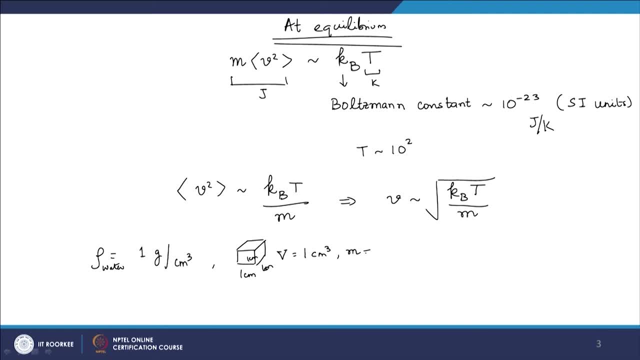 cube And therefore a mass of 1 centimeter cube multiplied by 1 gram per centimeter cube, that is 1 gram, that is 10 to the power – 3 kg in SI units, And if I now compute the temperature, that would be again. there are pre factors here. 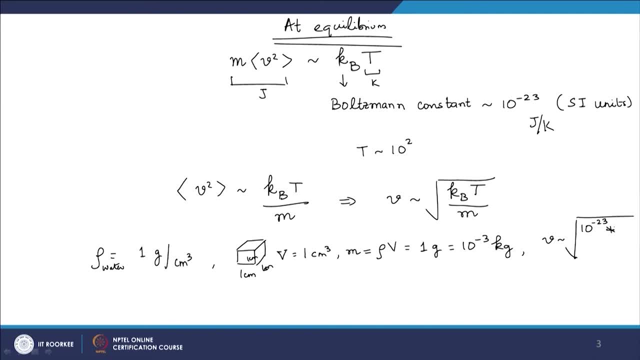 of the order of 1, but Kb goes like 10 to the power – 23, temperature goes like 100 and mass, in this case, is 10 to the power – 3.. So this gives me 10 to the power – 18 in SI units, that is meter per second, 10 to the 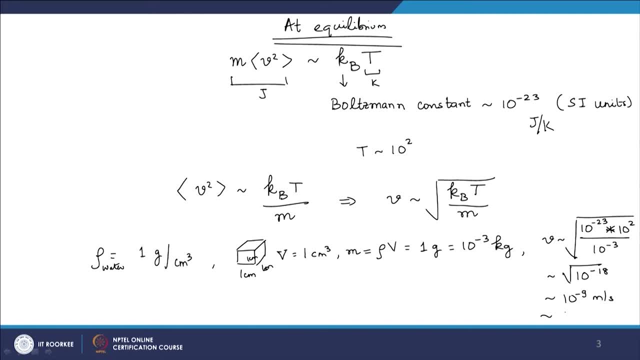 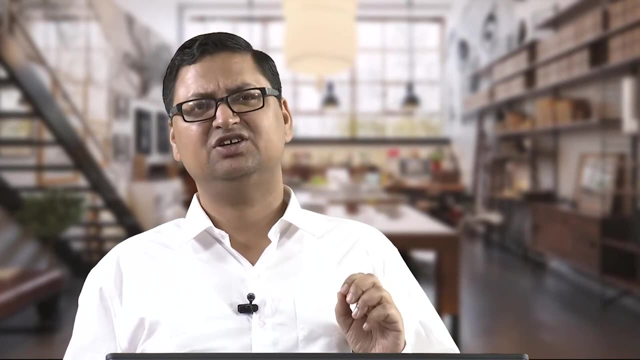 power – 9 meter per second. So if you have a 1 centimeter by 1 centimeter by 1 centimeter cubic block, because of temperature this would be moving at a velocity of 1 nanometer per second and the direction of velocity will. 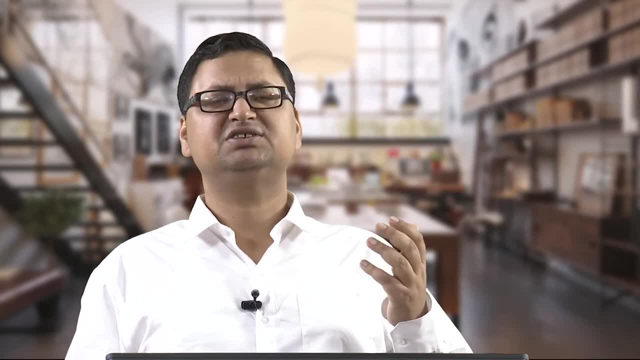 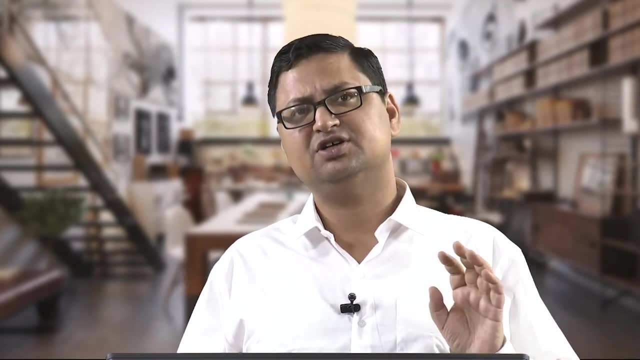 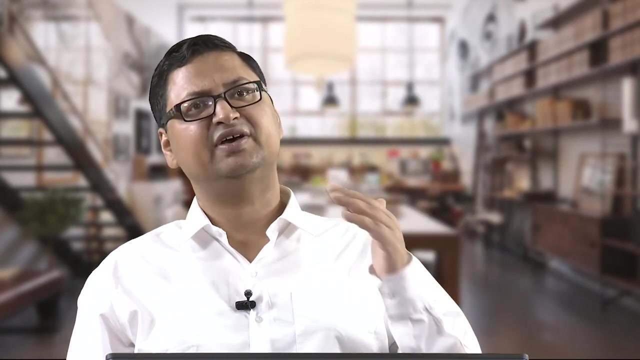 keep on changing with time because there is no external force being applied on the system. it is purely by diffusion. and diffusion can take place in different directions because other molecules come and collide on different occasions from different sides, and that is what is giving rise to the velocity that we see. 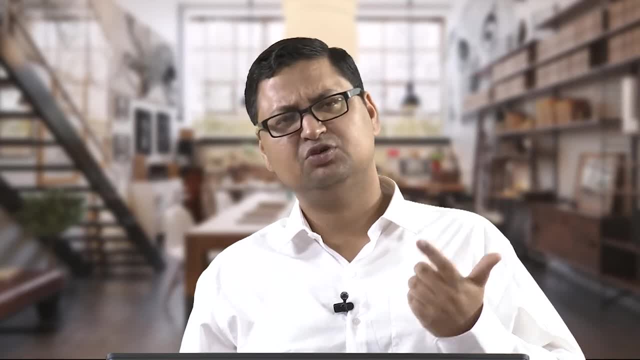 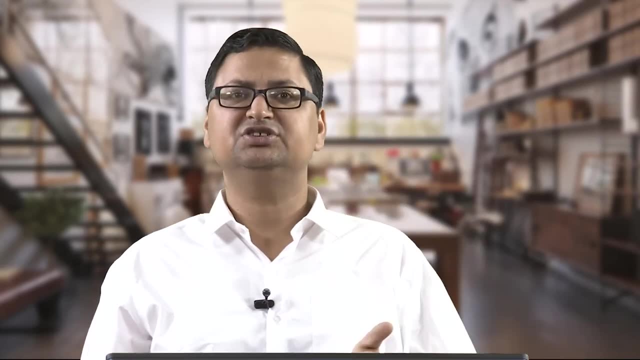 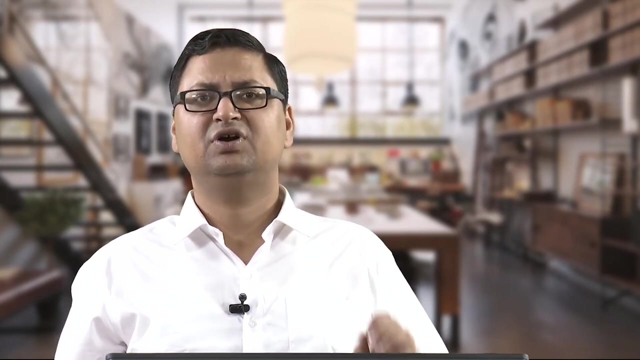 So 1 nanometer per second of velocity for a 1 centimeter cube block is almost negligible, provided also that it is not always in the same direction. it keeps on changing direction. So that is what the reason why we do not observe any sort of Brownian motion for large blocks. 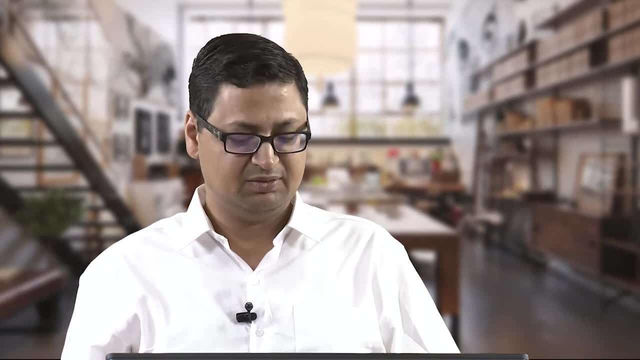 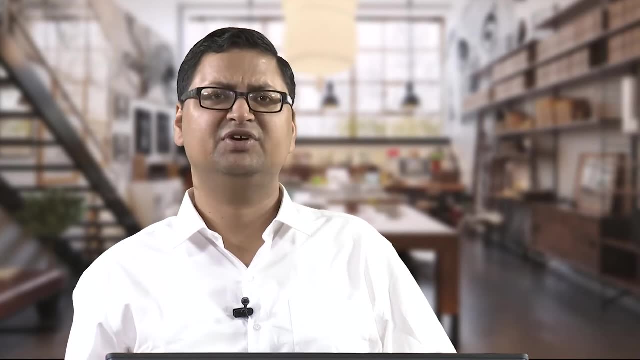 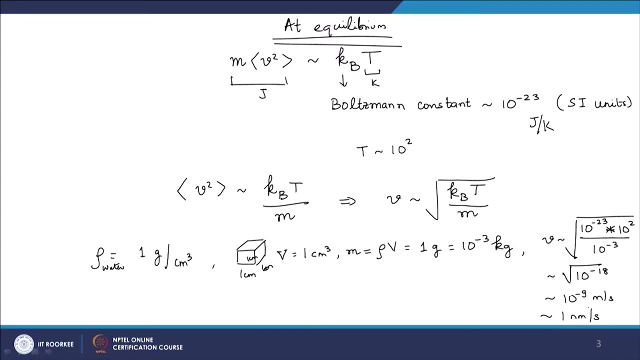 and if I think of say Ourselves, we are much longer than 1 cc, so our velocities because of Brownian motion will be even smaller and we can barely observe that. But if we really go to smaller systems, let us say now we look at a block that is 1 micron. 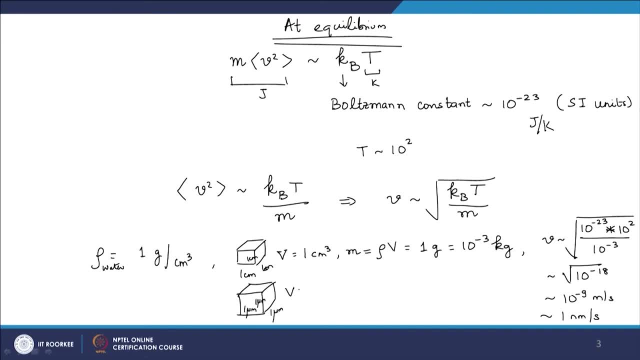 each. Now the velocity is 1 micron per second. Now the velocity is 1 micron per second. Now the velocity is 1 micron per second. Now the velocity is 1 micron cube and 1 micron is 10 to the power minus 4 centimeter. so 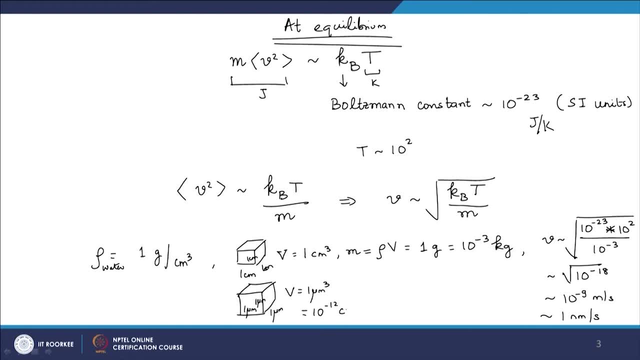 it is 10 to the power minus 12 centimeter cube. So now the mass will be 10 to the power minus 12 kg, and if I now look at the velocity, it is going to be 10 to the power minus 23 into 100.. 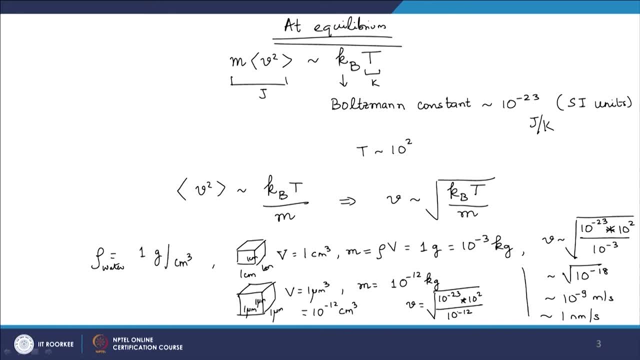 100 divided by 10 to the power minus 12, and this would be something like 10 to the power minus 9, which is of the order of 10 to the power minus 5 meter per second, which would roughly be like 10 micron per second. 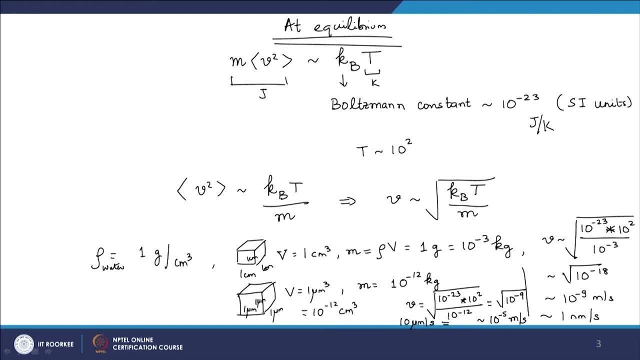 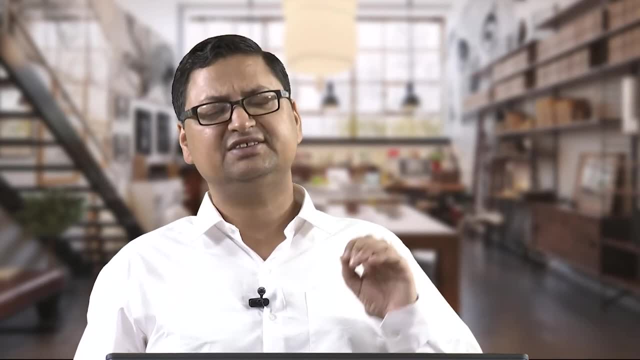 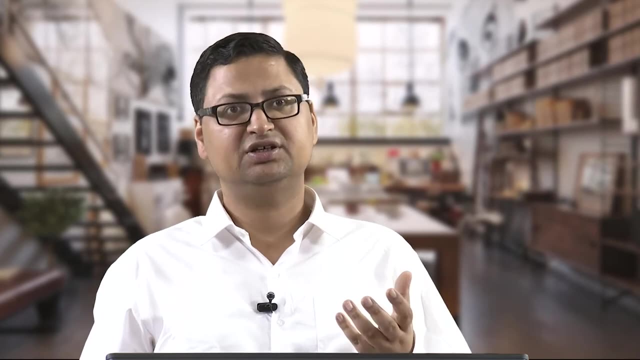 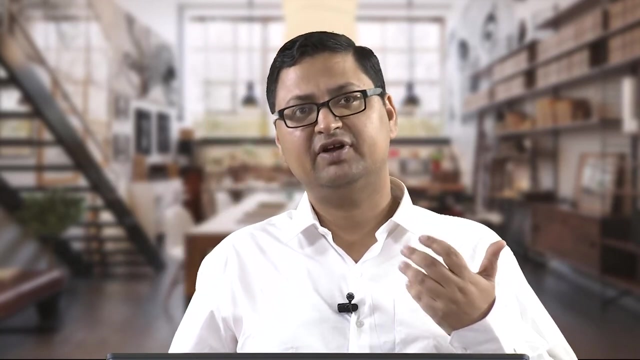 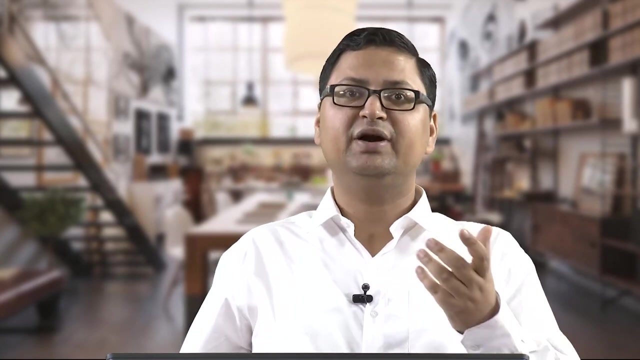 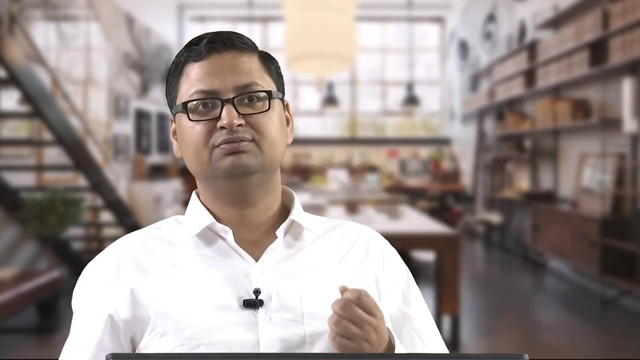 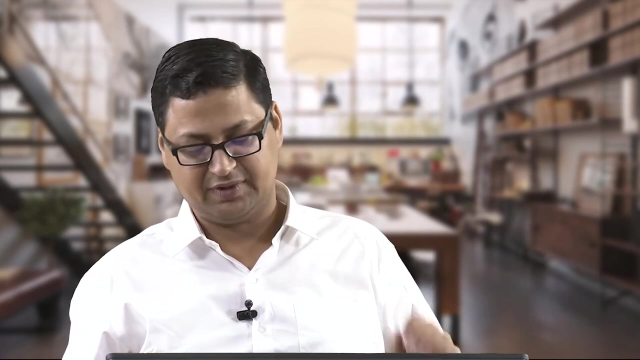 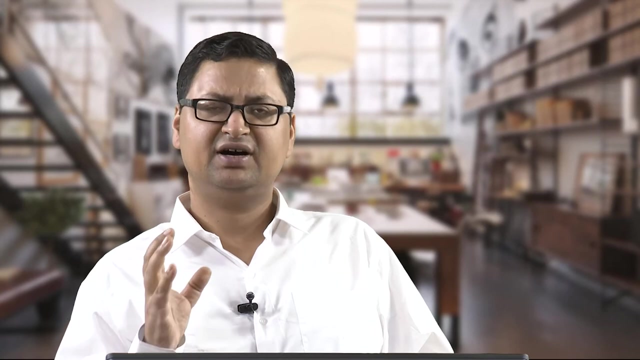 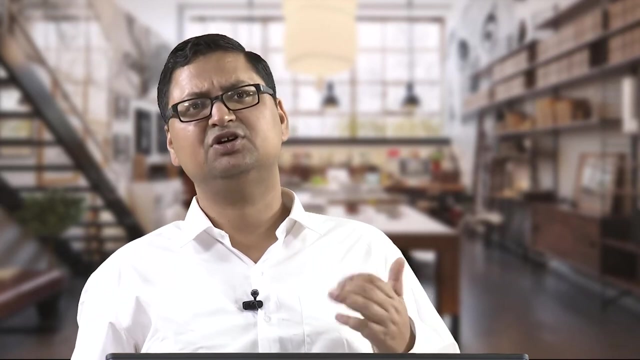 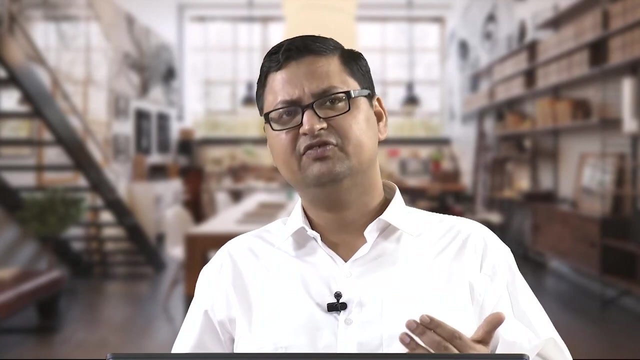 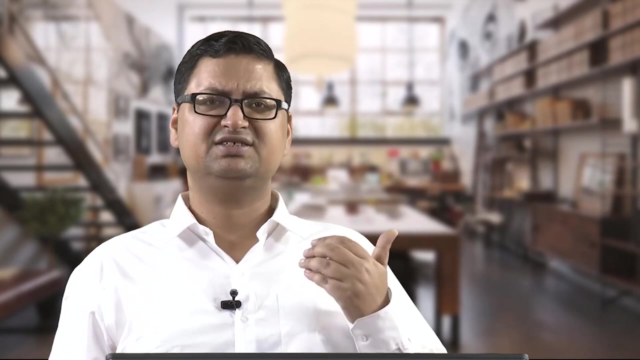 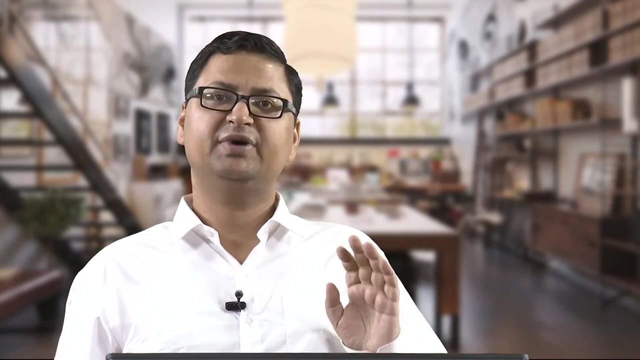 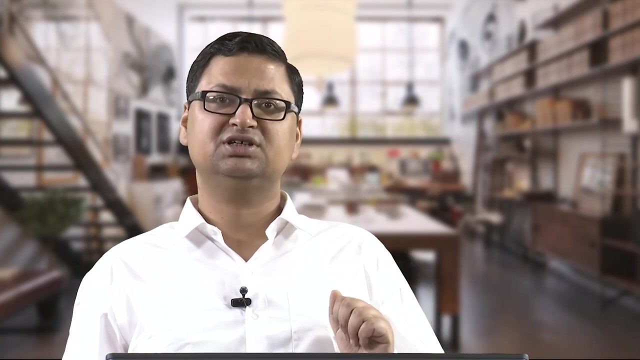 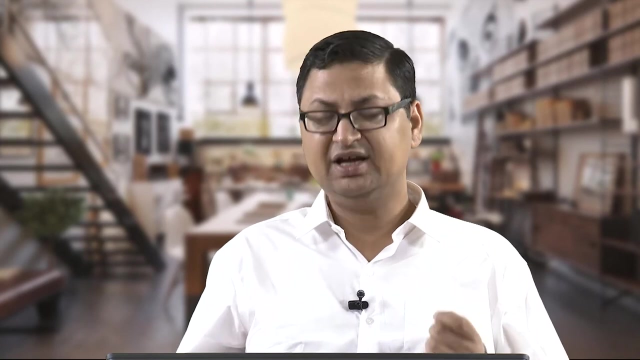 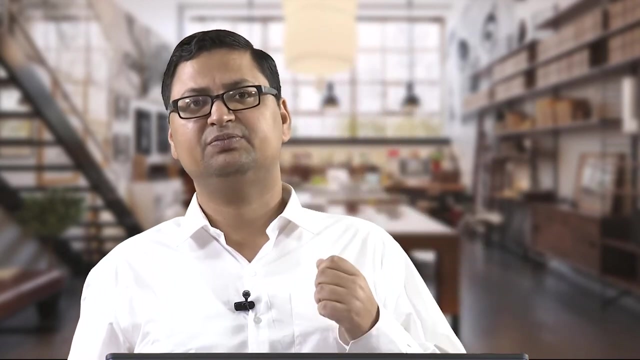 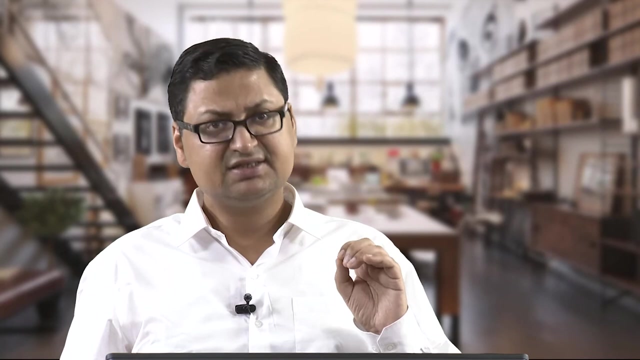 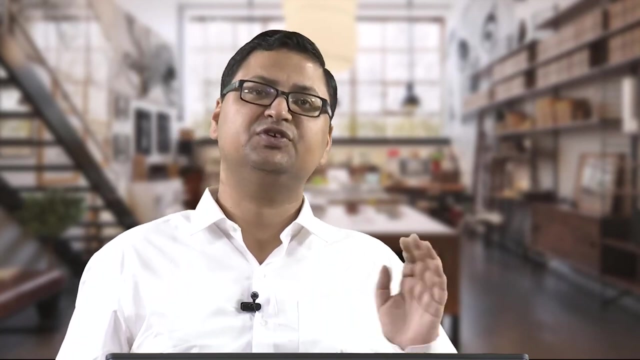 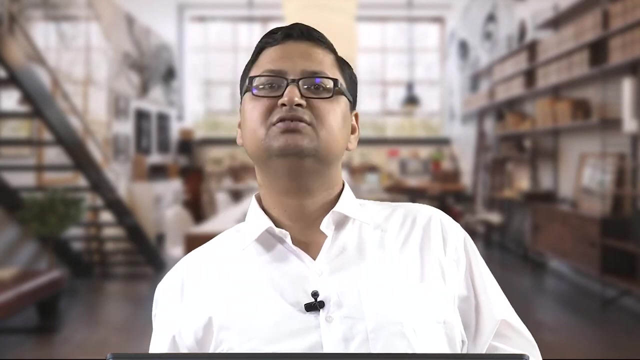 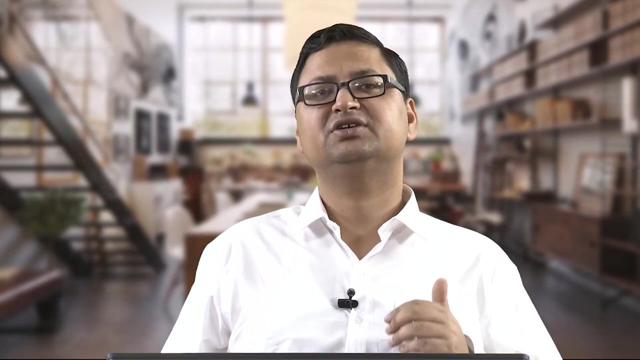 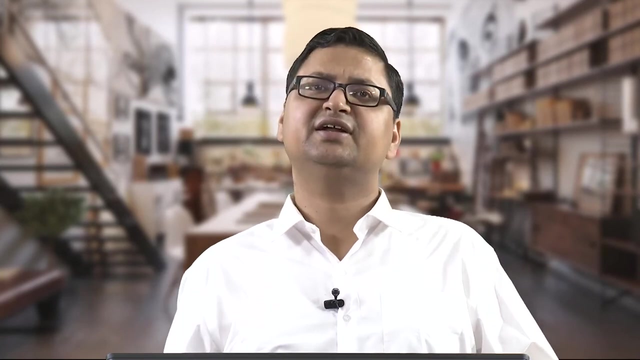 So these things tend to move from a high chemical potential to a low chemical potential. But the diffusion also exist for systems at equilibrium. the when we have, we do not have a real concentration gradient as such, because at the molecular level the molecules still 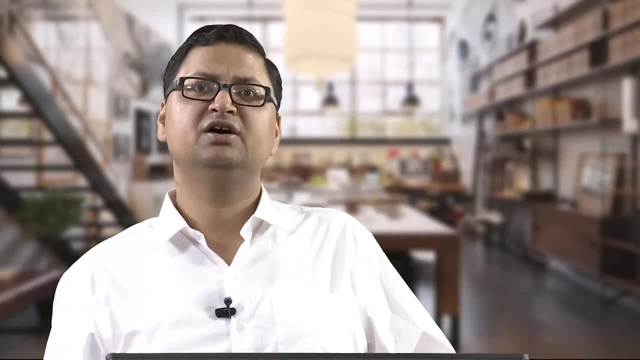 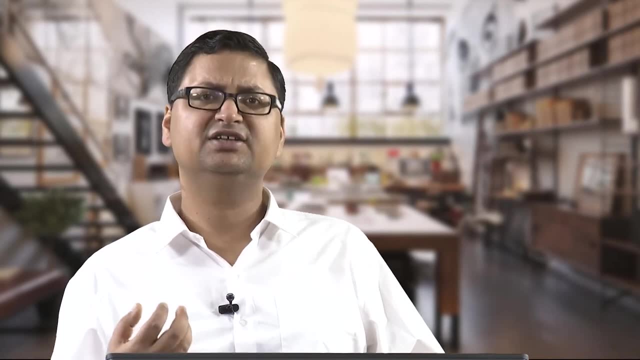 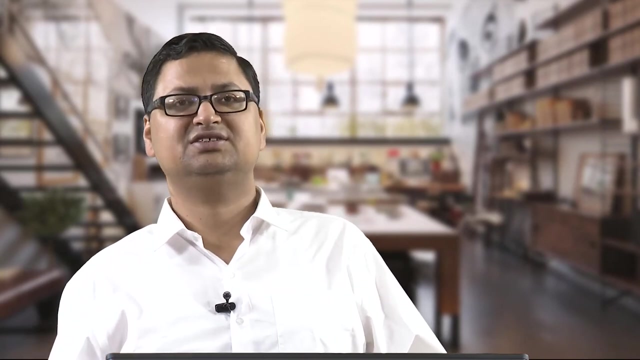 are undergoing collisions which are giving rise to this motion, especially in the case of a liquid and a gas. for a solid, it is rather difficult to visualize and these effects are typically negligible, Although, unless the temperature is 0 kelvin, we always have thermal energy in the system. 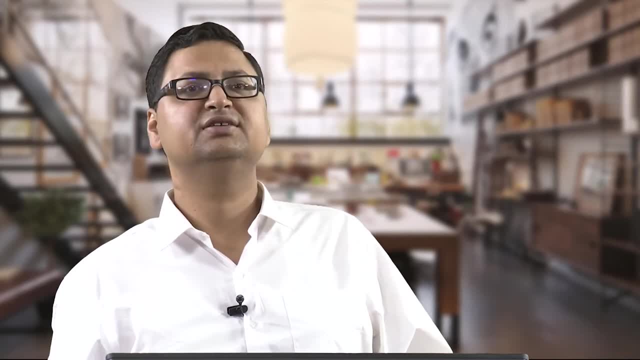 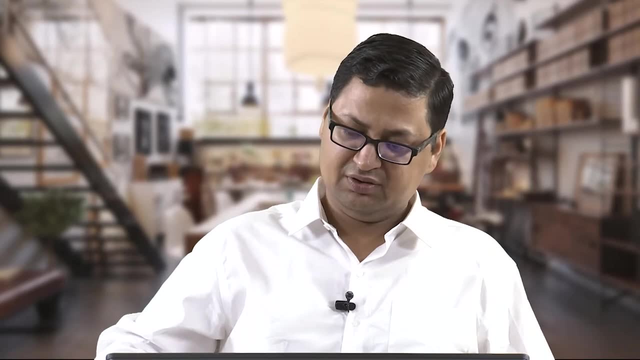 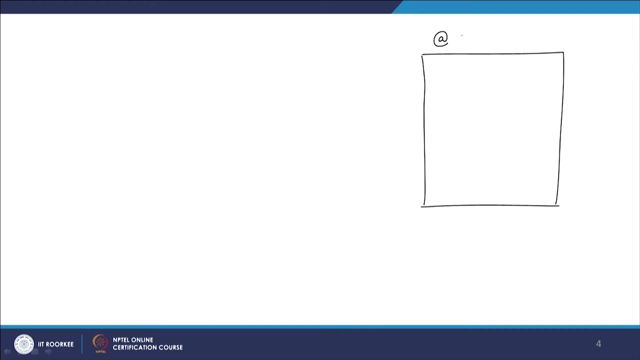 and thermal energy always is because of the collisions of molecules that are present in the system. Ok, so now, if I think of this kind of a movement happening at equilibrium, where each of the molecules are moving in different directions, the first thing we can 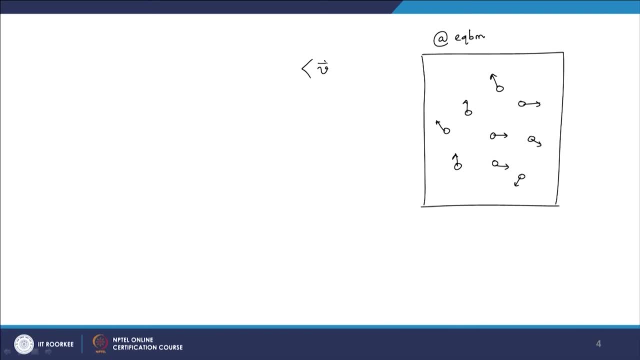 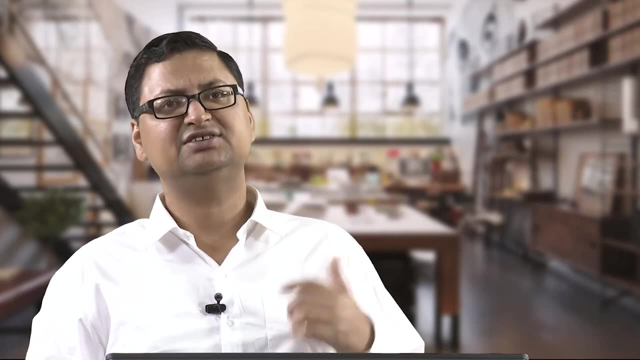 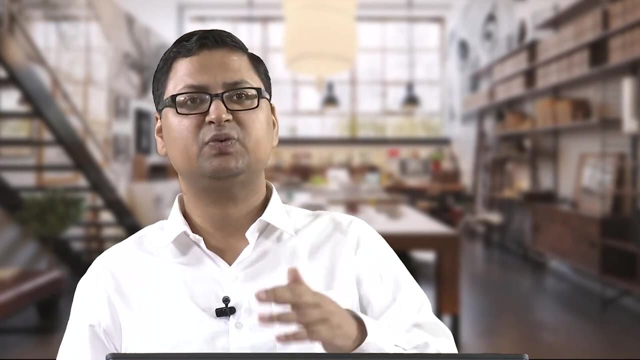 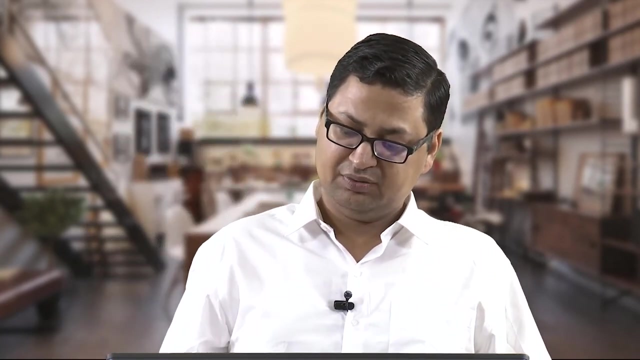 of course, note that the average velocity of the molecules need to be 0. Because there is net, no net movement in any direction. that is the reason why we used a mean square velocities in the previous derivation. that we just did, because the squares do add up, but the actual velocity is they cancel. and so if I look at any of the properties, 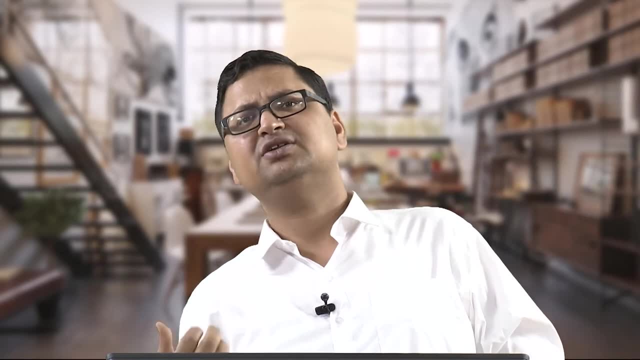 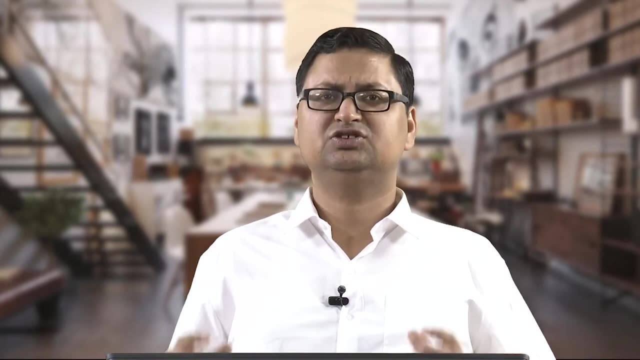 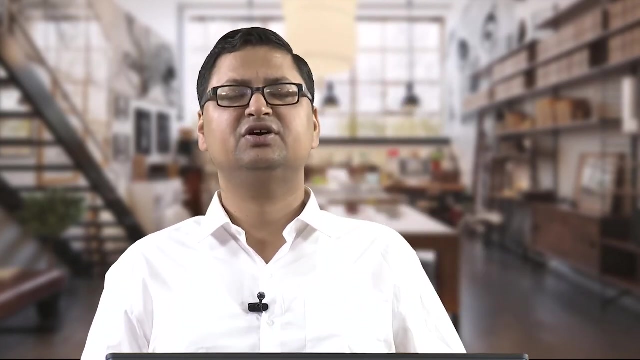 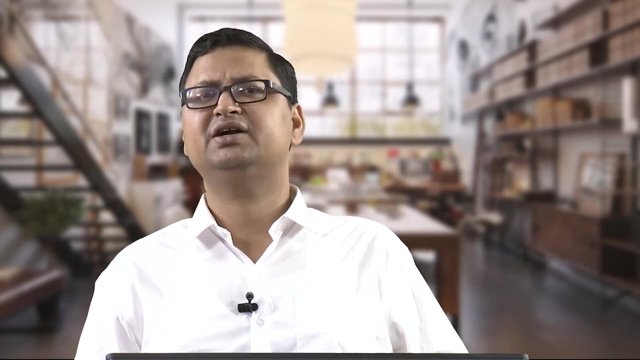 of this system. now, those properties also should depend on the this individual motion of each of the molecules and how they collide with each other, and so on. and since the collisions themselves are, although deterministic, because ultimately, if I know where the collisions are occurring, I can solve the Newton's laws of motion, I can get the position of particles, and so 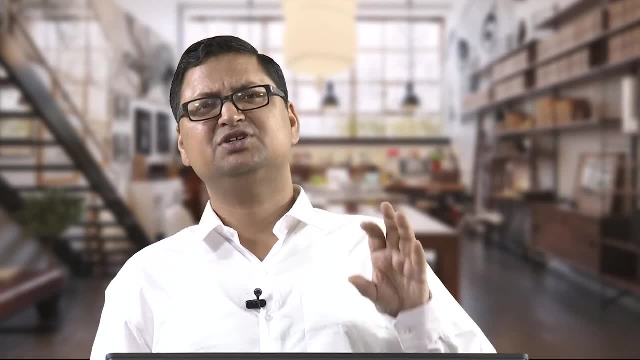 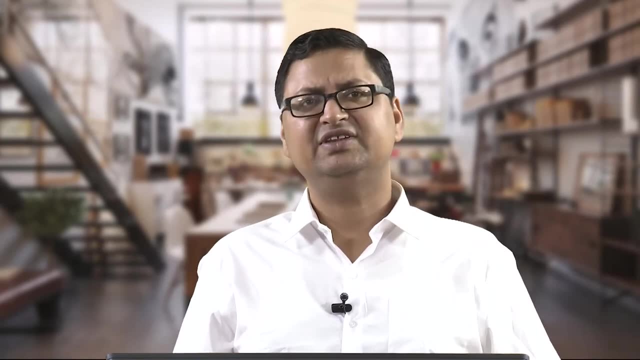 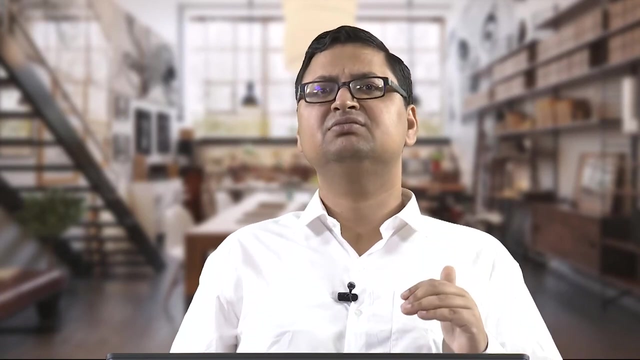 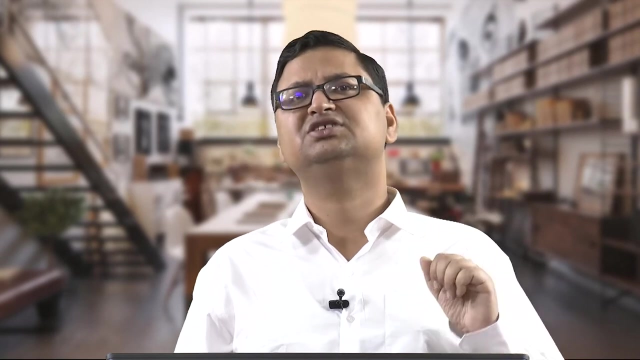 on. but since the number of molecules in the system is huge, it is very difficult to keep track of all the individual molecule in the system. What we then see is the properties of system tend to fluctuate because at any given time the configuration of molecules and the velocity of molecules are not constant. they are continually. 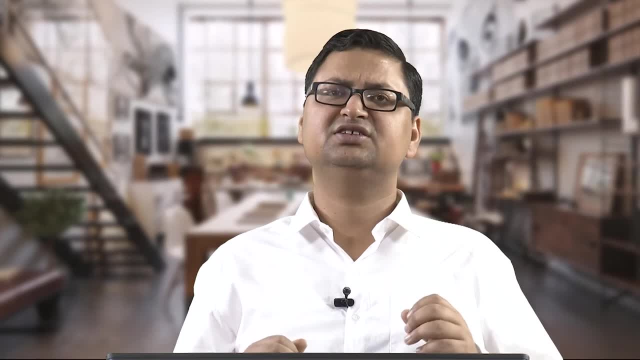 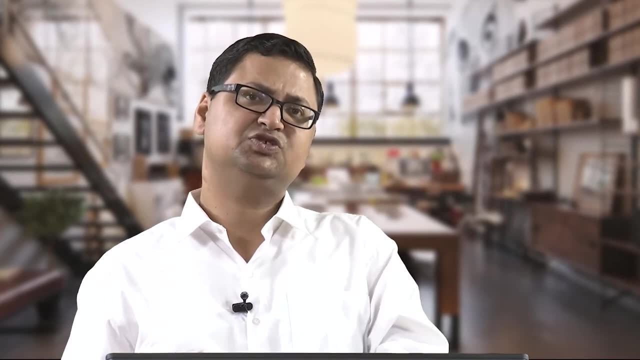 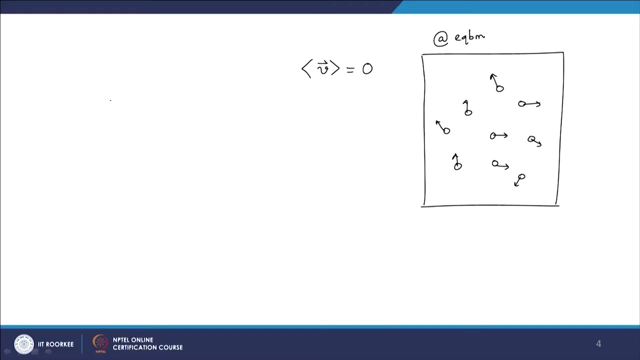 changing, and different configuration means different orientation of molecules, different velocity of molecules With give rise to fluctuations in the property of the system. let me see, even at equilibrium, ok. So, and I am talking about any thermodynamic property here, it would appear to us that any. 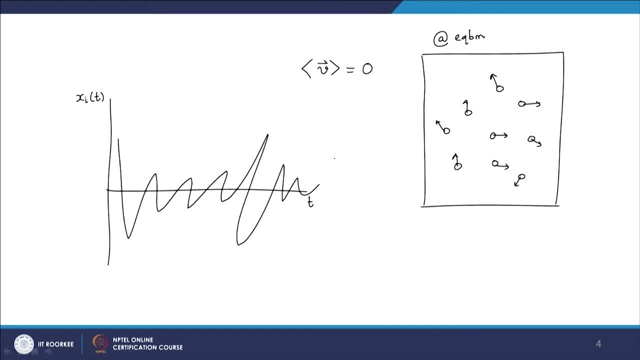 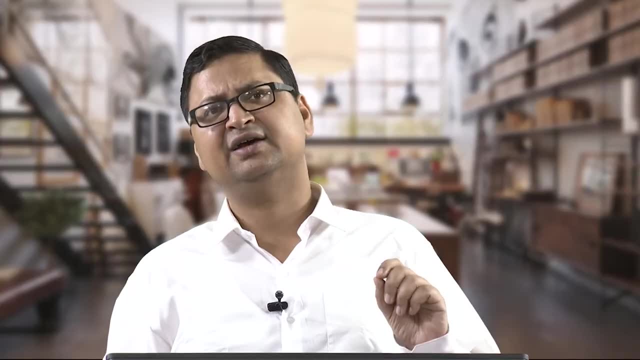 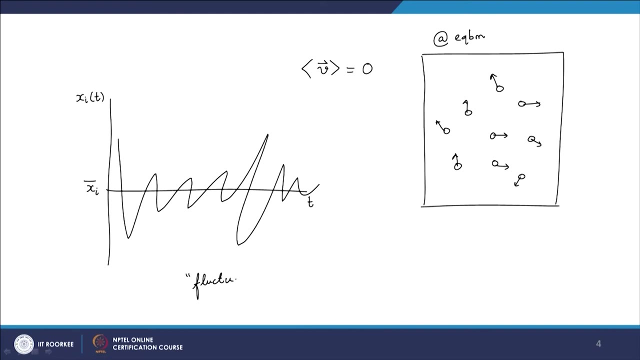 quantity we look like tend to fluctuate around some mean value. let us call it xi bar. but I want to note again here that the fluctuations are not random, although you will see that I will use a random function to characterize the fluctuation, purely for mathematical reasons. 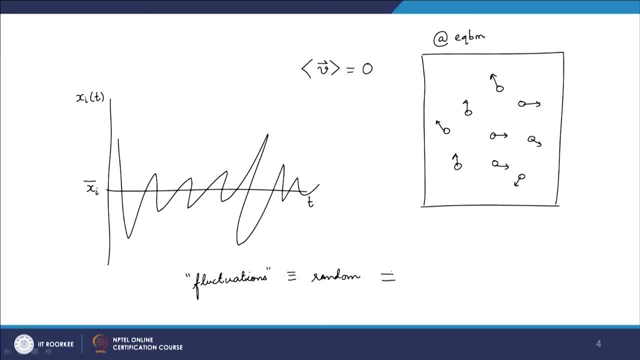 fluctuations are not random. they are simply a result of the fact that molecules have different velocities at different times because of the frequent collisions it is having with other molecules in the system. ok, So in principle it is fully deterministic. So, in principle it is fully deterministic. 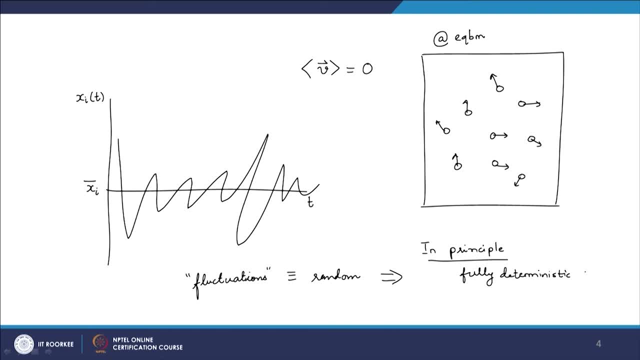 if that is a big, if we can solve equations of motion of all molecules. So over the time, what we should see if this molecule, let us say it has start going in this way, undergoes a collision, changes direction, undergoes collisions again and again. it has certain trajectory. 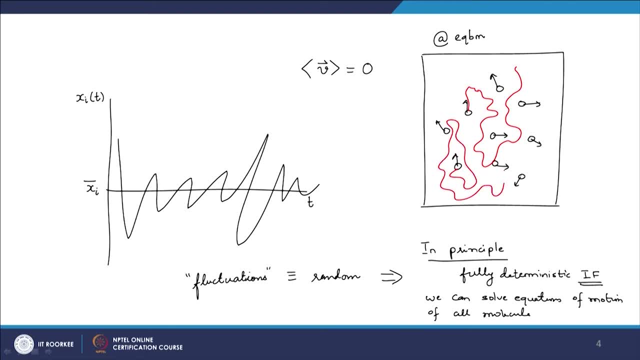 Similarly, other molecules will also undergo collisions, change direction, will have certain trajectory and if we can really do solve the equation of motion, We can get the trajectory of all the molecules. and this is what essentially what we do in a molecular, How dynamics, simulation. the only limitation is it is for very small system, let us say simulation. 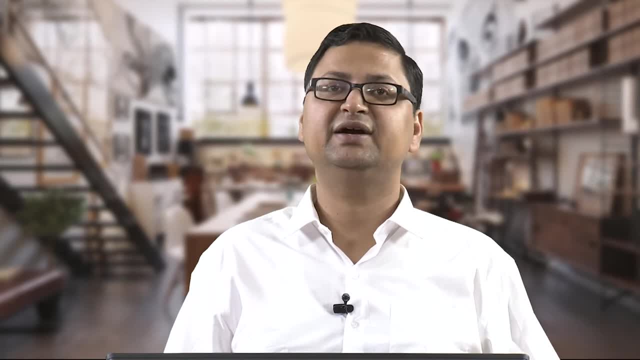 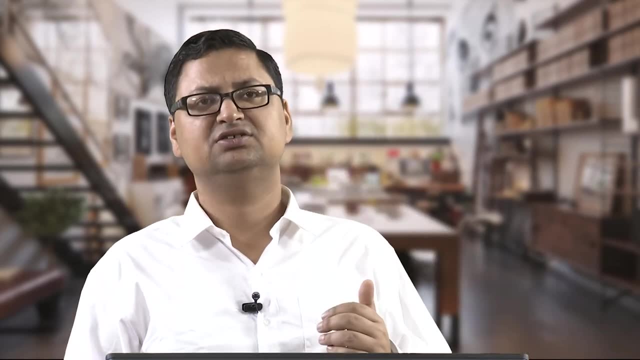 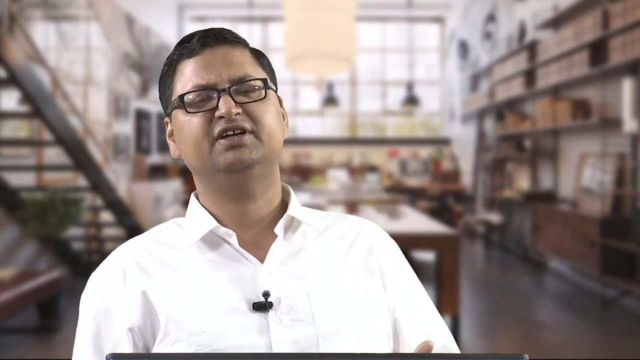 box of the order of 10 nanometer by 10 nanometer by 10 nanometer For larger systems, we will have molecules in millions of molecules and it is very difficult to keep track of trajectories of all the molecules. and do that and there is an easier approximate. 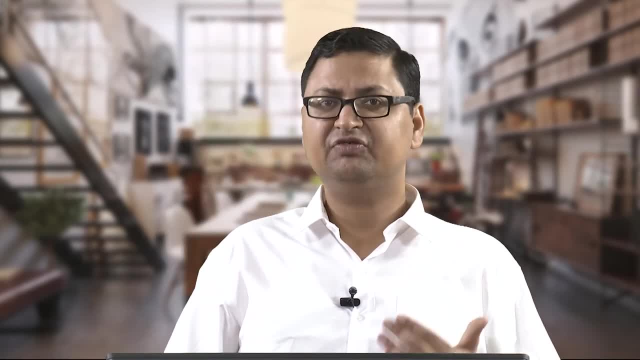 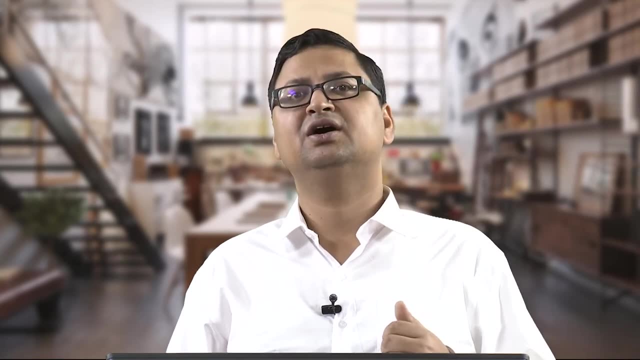 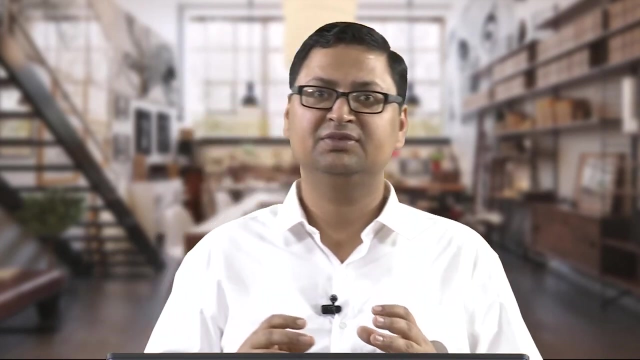 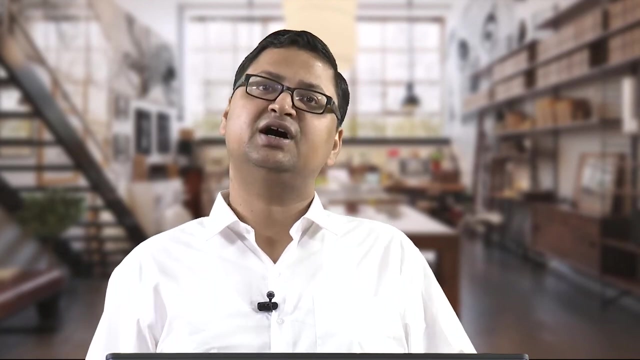 way that tells me about the behavior of the system, assuming that the fluctuations are somewhat random, purely again in mathematical terms. I want to emphasize this point over and over, that the process is not random, but we use a random function to characterize the process and the final outcomes are somewhat such that they make physical sense. 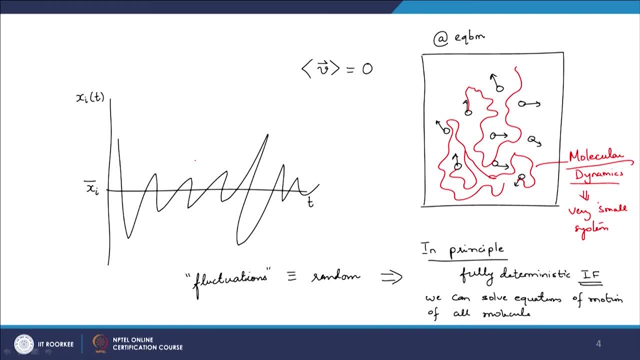 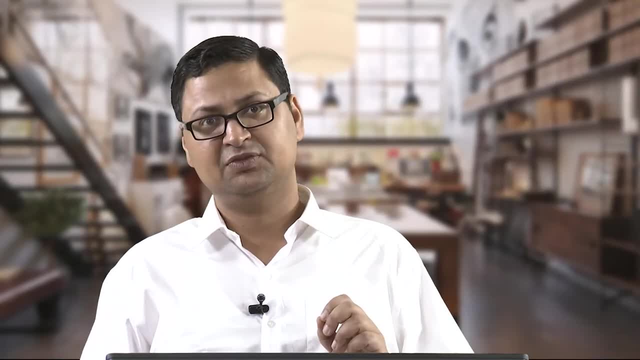 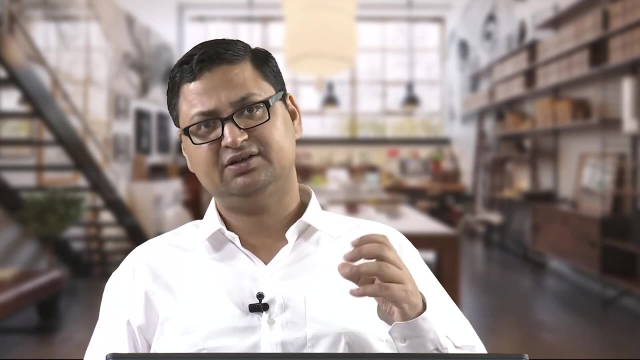 So if you do see a property, it shows fluctuations like this, and then, of course, the mean values is what we typically are interested in. but to characterize the magnitude of these fluctuations- because those magnitude actually are a result of the Brownian motion- we will use what is. 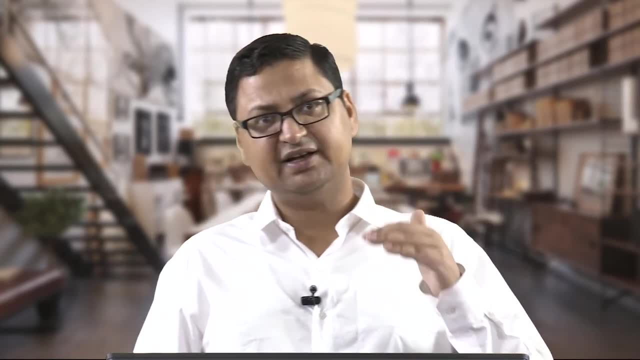 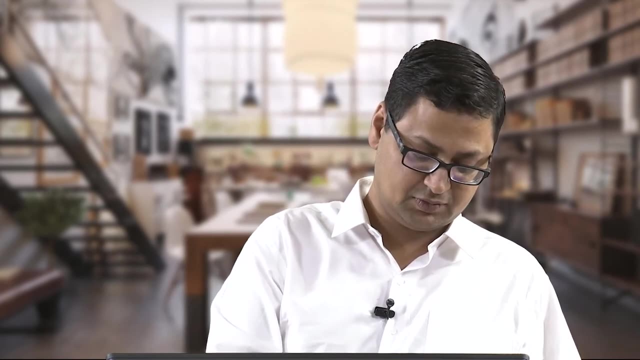 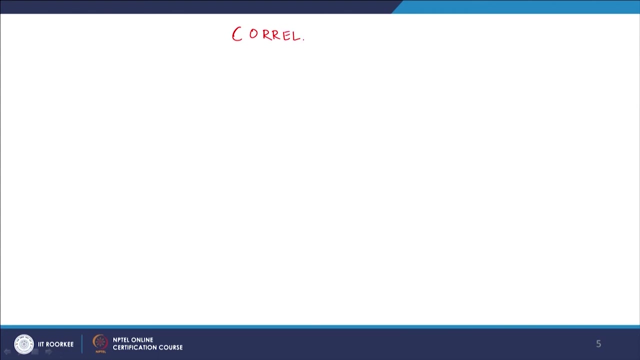 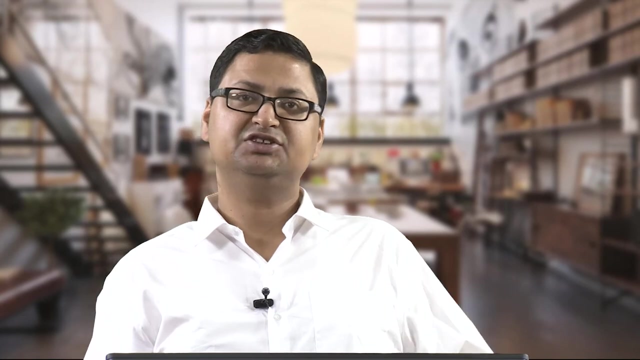 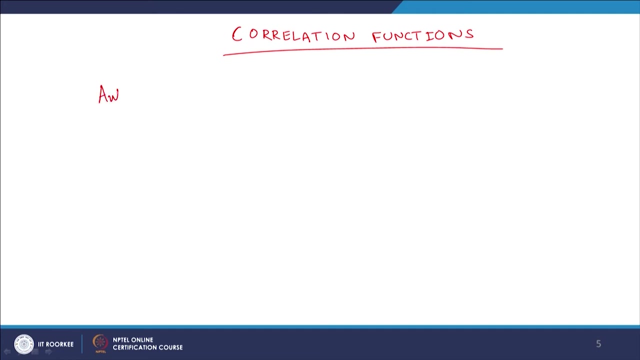 known as correlation functions. that characterizes the magnitude of fluctuations, not the average value. property right. So we will use correlation functions, and there are two different correlations functions I will use to characterize the magnitude of Brownian motion. One we call An autocorrelation function and other we call a cross correlation function. 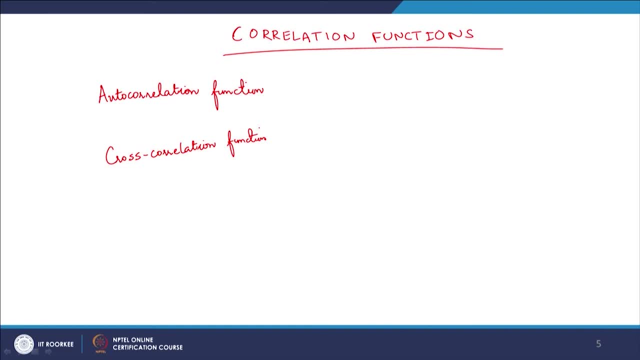 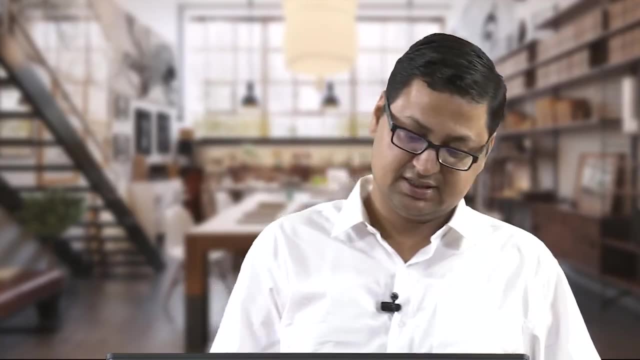 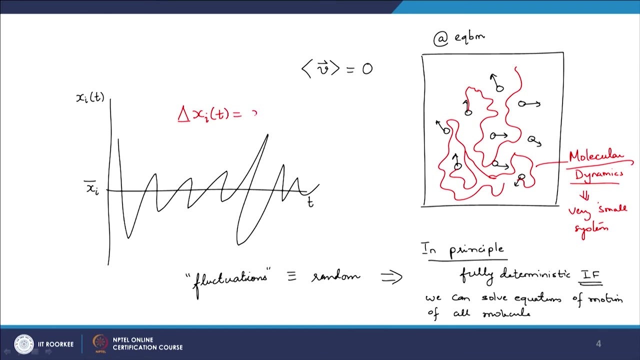 and for both of these it is preferable that, instead of looking at the actual, The actual value of the property, what we look at is some sort of deviation from the mean value. let us say mean value we have already computed or we know from experiment we take. 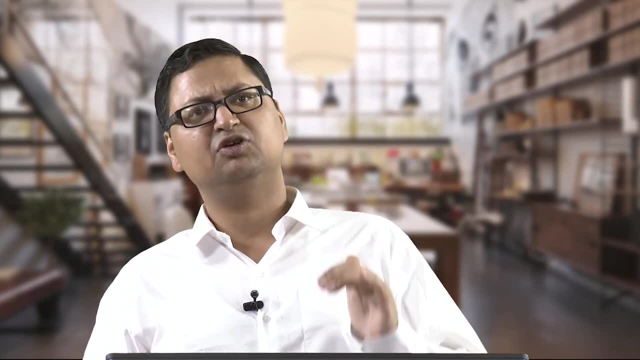 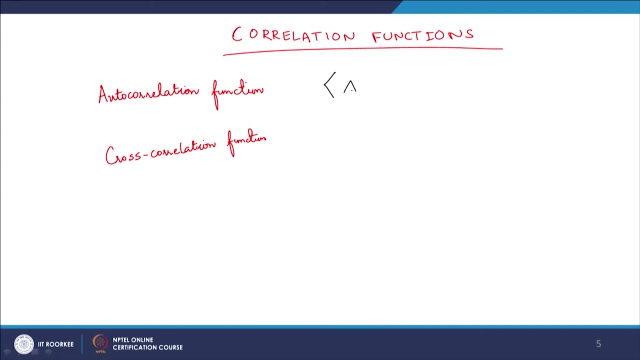 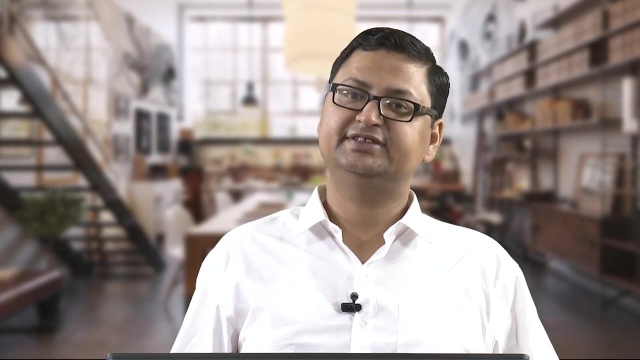 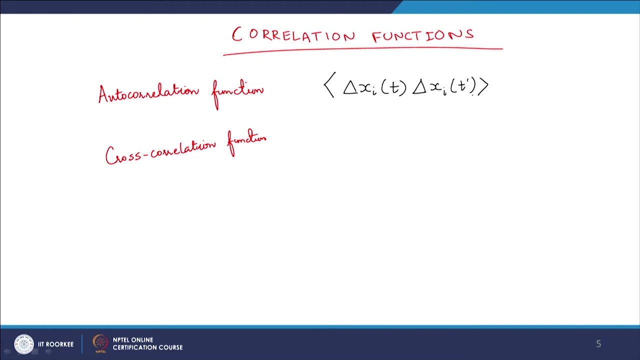 the deviation from the mean value, and this characterizes the amount of fluctuation at a given time. So autocorrelation function Is defined as delta of x i t. autocorrelation function is defined for the same property as delta x i t and delta x i t prime. that characterizes the magnitudes of fluctuations. 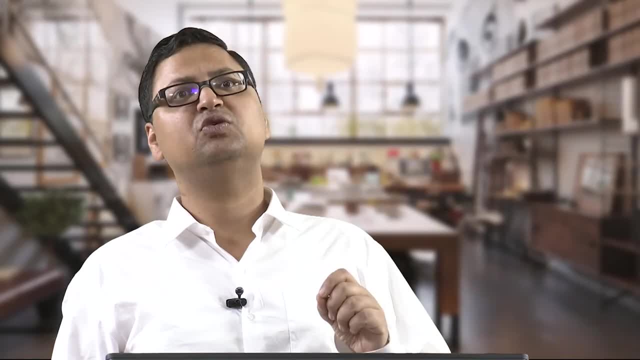 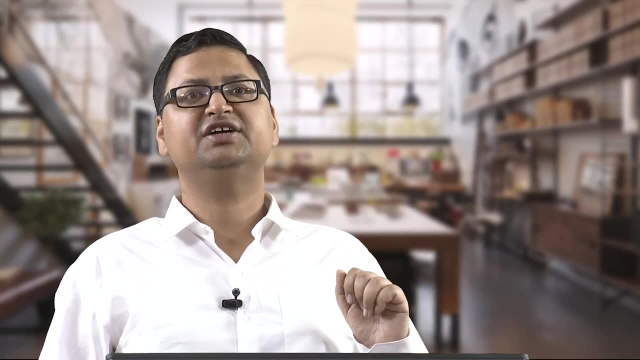 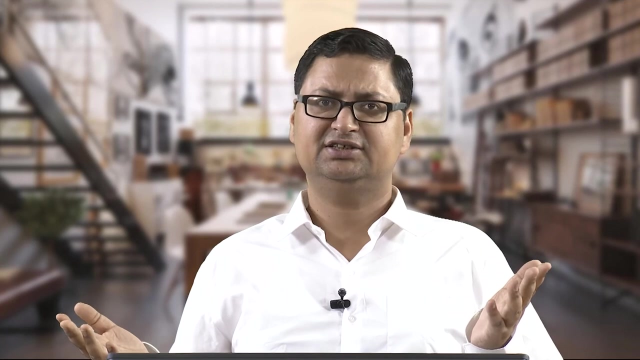 at two different time point, time points- and how are they correlated? So if it is completely a random process, then the deviation we have at any time and any time else they should be completely uncorrelated. so let us say, if I am doing a coin toss experiment, 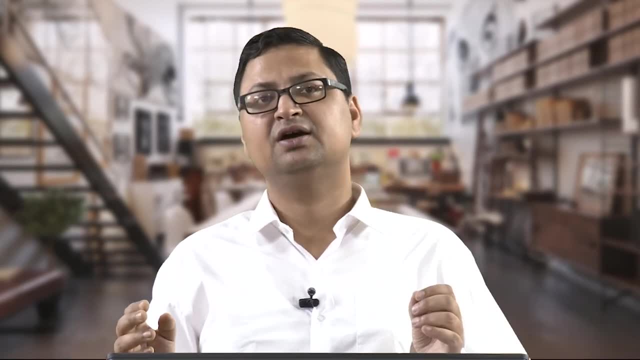 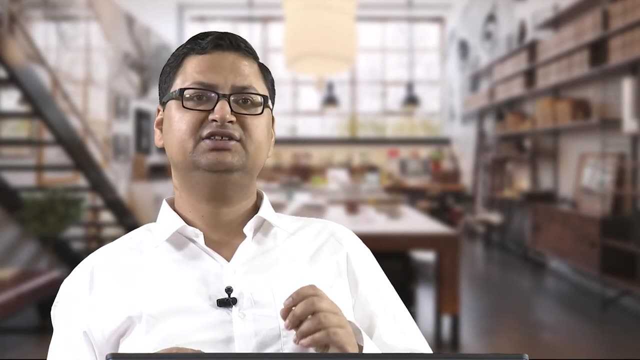 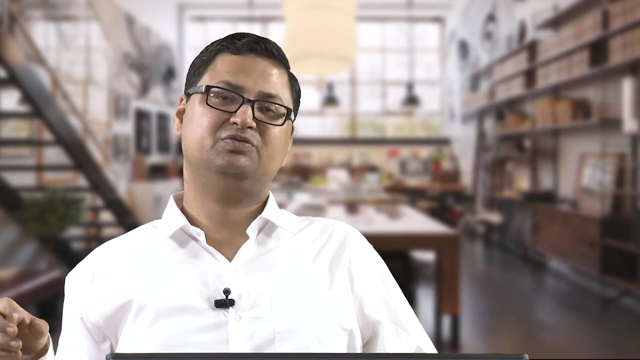 each of the event is completely independent of the other, but if I think, in terms of the Brownian motion, the immediate events are correlated and even the events after are correlated because the particle is undergoing a trajectory. the new position of particle of course depends on the old position. of course the correlation may decay with time, but the correlation is.